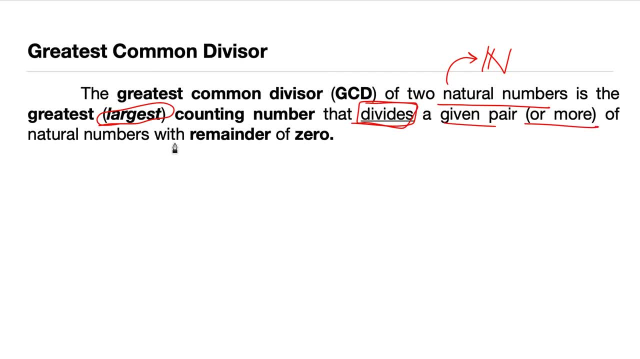 okay, take note. divides a given pair or more numbers of natural numbers into remainder of zero. okay, divides them completely with a remainder of zero. So both of them, or all of them, must have a remainder of zero, that is, they're completely divisible. The greatest common. 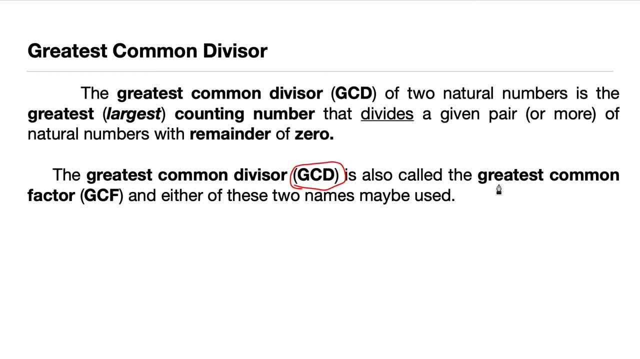 divisor, also known as GCD, is the greatest common divisor, also known as GCD, of two natural numbers. for shorthand is also known as, or also called as, the greatest common factor, or actually in the UK they call that as HCF or highest common factor, And either of these two names or three. 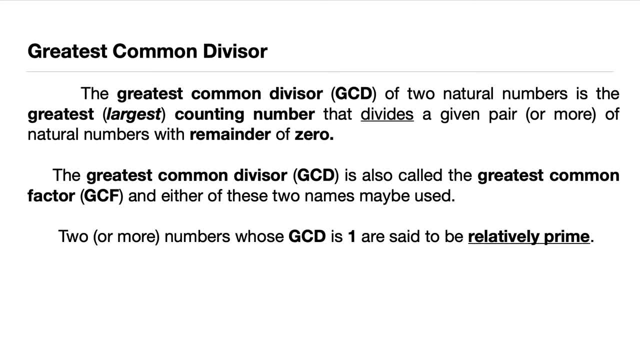 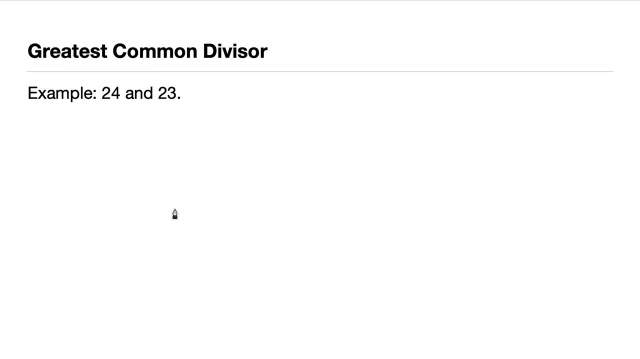 of these names can be used Two or more numbers whose GCD or greatest common divisor is one is said to be relatively prime to each other. Okay, so, for example. so say, for example, we have here 24 and 23.. So how can we get the greatest common divisor or GCD of 24 and 23?? What we need to do first is: 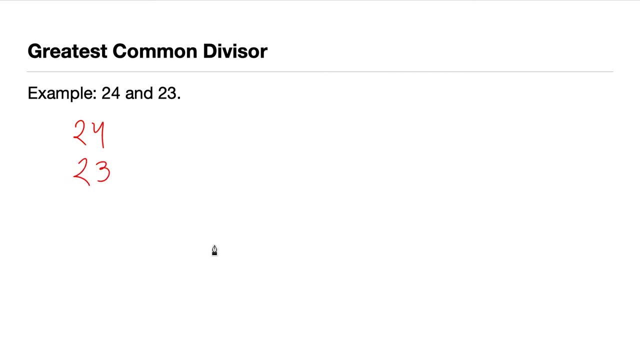 to prime factorize both of them, prime factorize both of them. So for 24, we know that let's use the factor three in this instance. So this is 2 times 12,. okay, 2 times 12.. And we have this is. 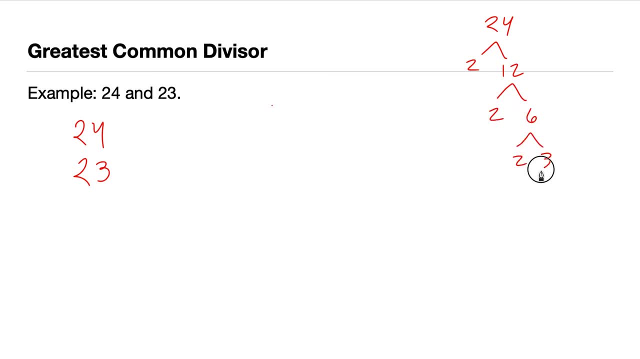 going to be 2 times 6.. And then, lastly, 2 times 3.. So how do you write this? This is going to become times 2 times 2 times 3.. And how about for 23?? Actually, 23 is a prime number, so it has only 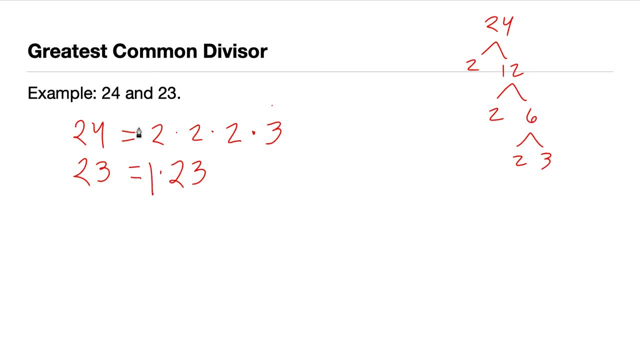 one pair, 23 times 1.. Actually, 1 is trivial. It should be always as a factor. So, as you can see here for 24 and 23,, it has only one similar or common divisor, which is 1.. So from this example, 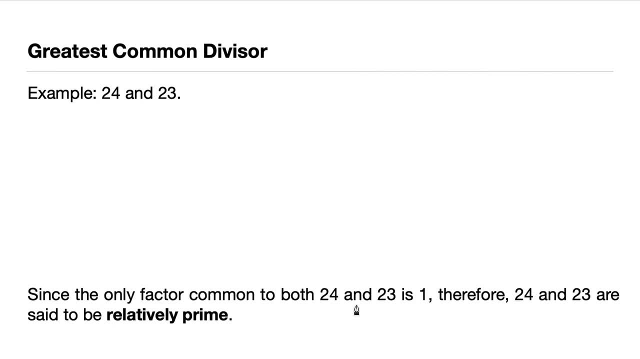 we can say that, since the only factor of both 23 and 24 is 1,. therefore we say that both of them are relatively prime to each other. They are relatively prime since they have only 1 as the common factor. So that is what you mean when you say it's relatively prime. Let's have another. 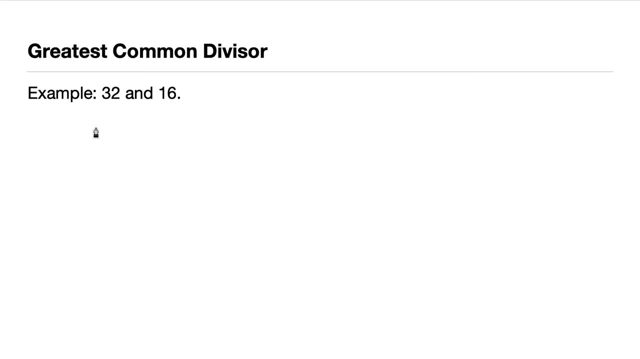 example, shall we? So let's have 32 and 16.. So how do we get the greatest common divisor, 32? And 16.. So let's factor 32 first, using the factor 3.. So we have 32.. Let's divide this by 2,. 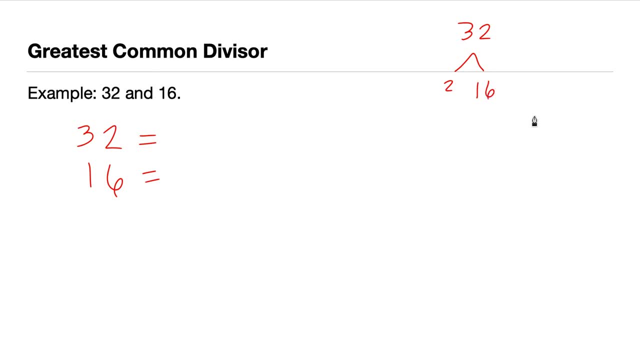 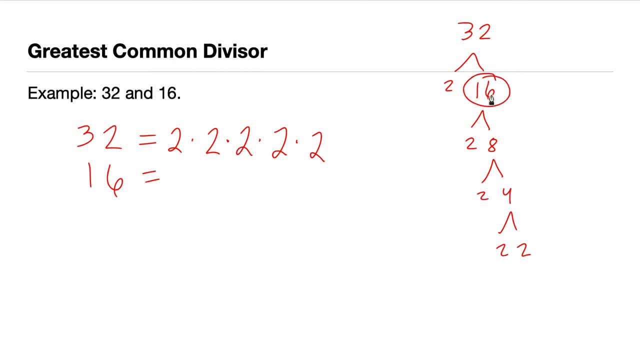 1, 2,, 3,, 4, 5.. And 16, we can see 16 over here, So we can just follow the rest here. So this is going to be 2 times 2 times 2 times 2.. Now how do we get the greatest common divisor of these two? 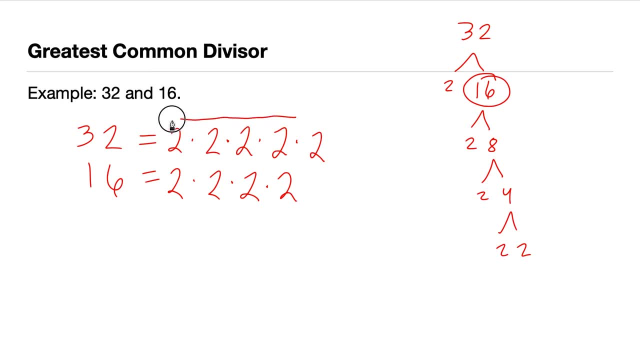 numbers. What we need to do is just box the numbers which are common to both of them- Again, common to both of them- And we can see that these are these numbers. These two is just outside the box because there's no common divisor. So we can just box the numbers which are common to both of. 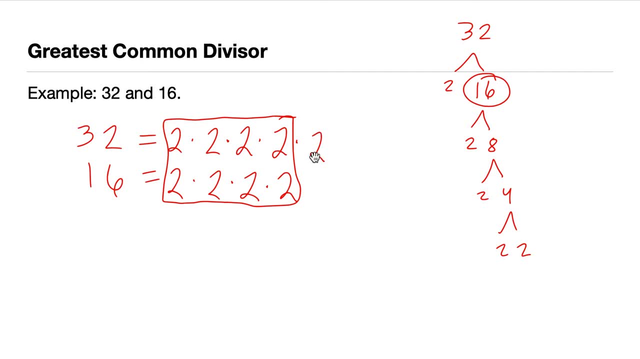 them. So external 2, the 16.. So this is not common. This is number 2, this integer 2.. It's not common to 32 and 16.. So what we will do is the common factors are, say, the common factors. 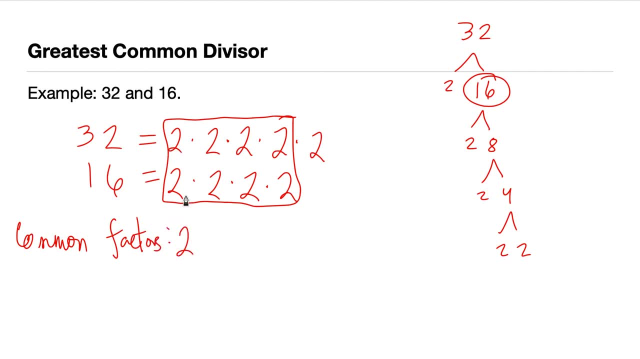 are. let's write it down: You have 2 times 2 times 2.. Since we have four integers which are common to them. So therefore we can say that the GCD of the two numbers, then the GCD, GCD of 32 and 16, is of both numbers. shall we say.